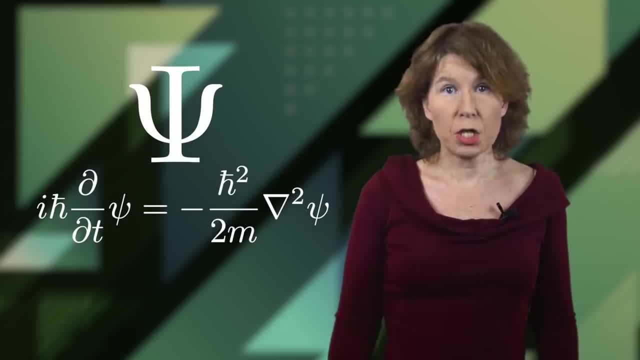 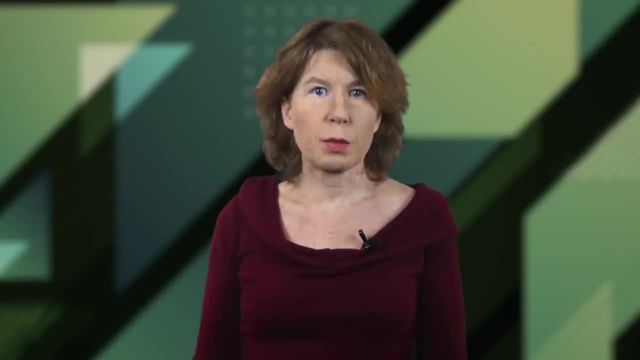 reading an equation, But the wave function itself isn't measurable. Instead, from the wave function you just calculate probabilities for measurement outcomes. Quantum mechanics might, for example, predict that a particle hits the left side or the right side of a screen with 50 percent probability. 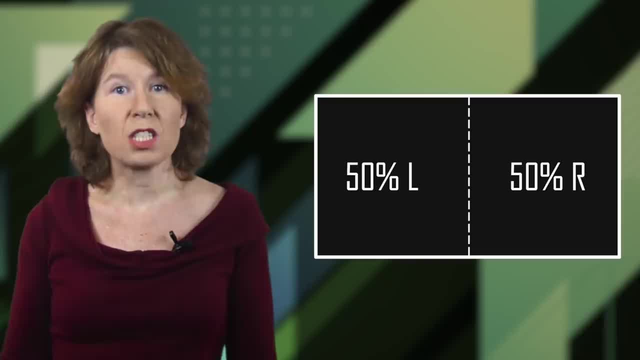 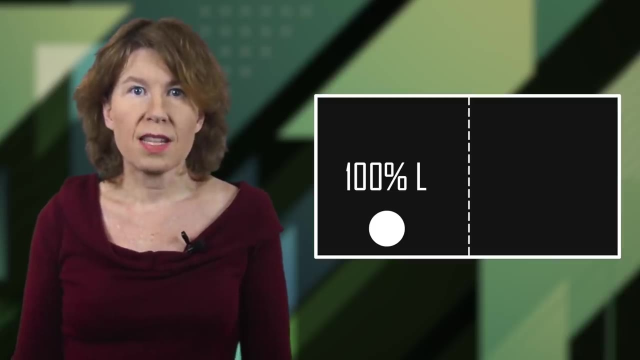 each. Before the particle hits the screen, it is in a superposition of those two states, which means it's neither here nor there. Instead, it's in some sense both here and there. But once you have measured the particle, you know where it is. with 100 percent probability, This means 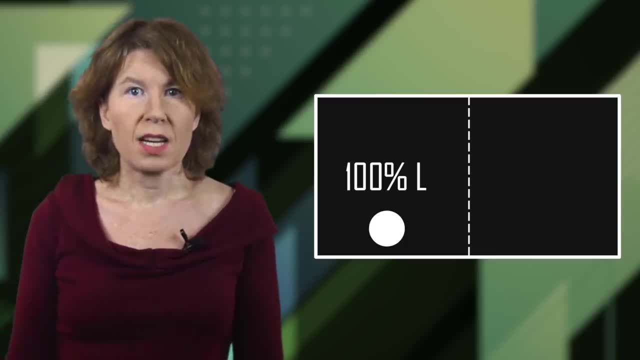 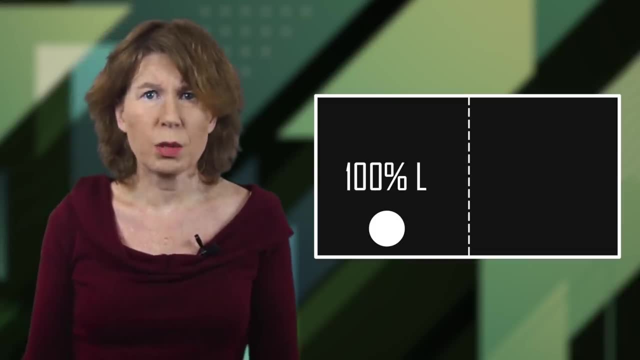 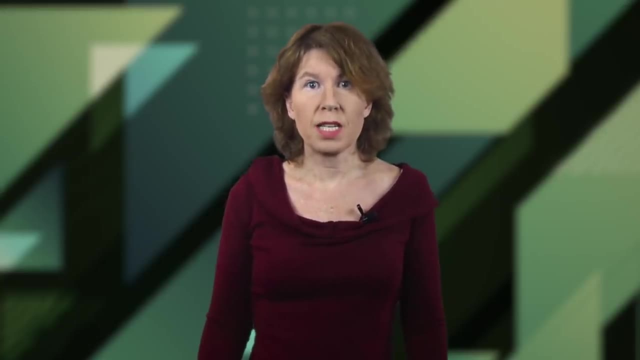 after a measurement, you have to update the wave function. This update is also called the reduction or collapse of the wave function. What is a measurement? Quantum mechanics doesn't tell you, And that's the problem. Wigner illustrated this problem with a thought experiment, now known as. 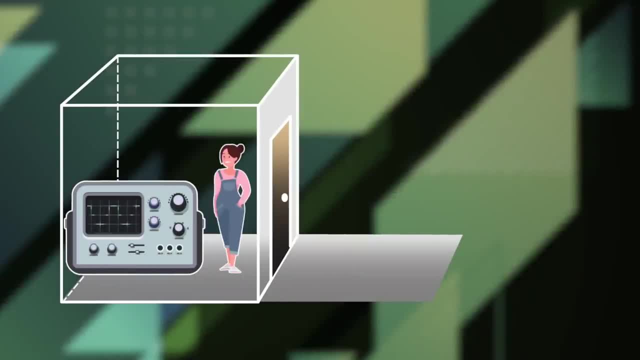 Wigner's friend. Suppose: Wigner's friend Alice is in a laboratory and does an experiment like the one we just showed you. This experiment is called the Wigner's friend. Alice is in a laboratory and does an experiment like the one we just showed you. Alice is in a laboratory and does an experiment. 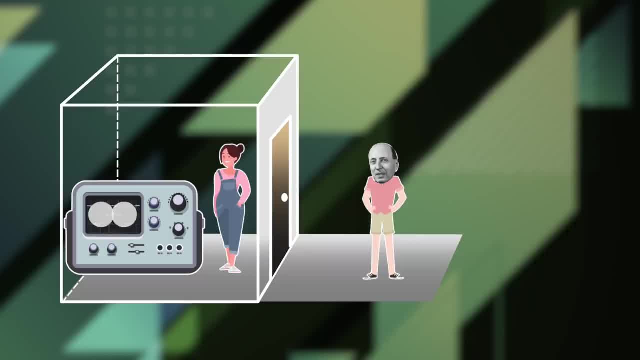 talked about. Wigner waits outside the door. Inside the lab the particle hits the screen with 50 percent probability left or right. When Alice measures the particle, the wave function collapses and it's either left or right. She then opens the door and tells Wigner what she's. 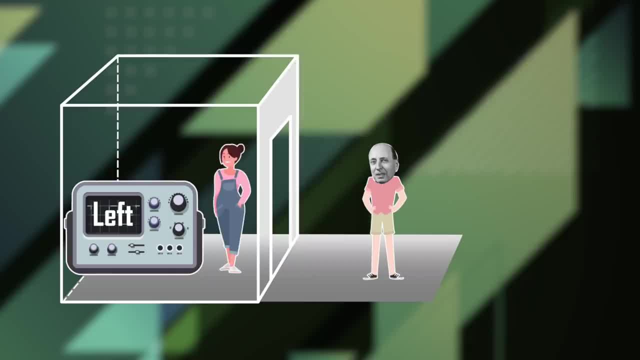 measured. But how would Wigner describe the experiment? He only finds out whether the particle went left or right when his friend tells him. So, according to quantum mechanics, Wigner has to assume that, before he knows what's happened, Alice is in a superposition of two states, one in which the 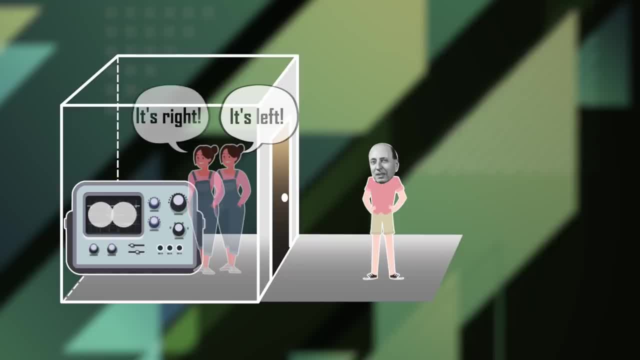 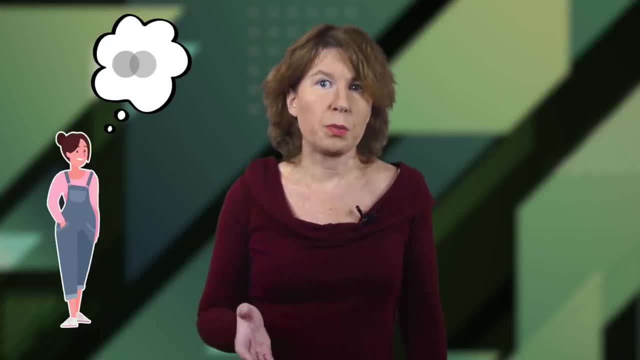 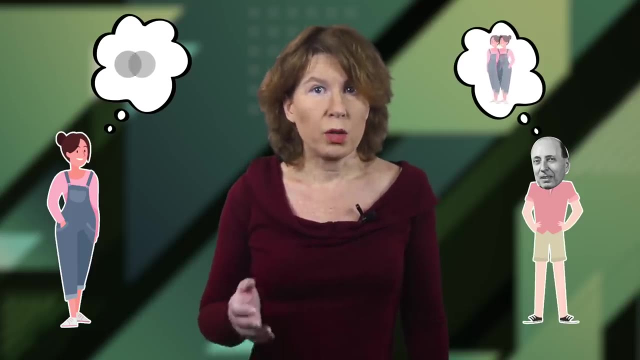 particle went left, and she knows it went left, and one in which it went right, and she knows it went right. The problem is now that, according to Alice, the outcome of her measurement never was in a superposition, whereas for Wigner it was, So they don't agree on what happened. Reality. 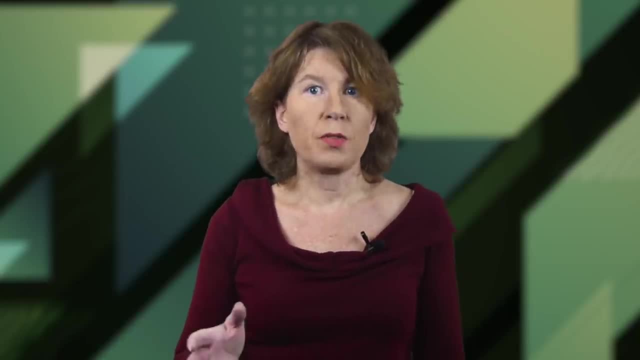 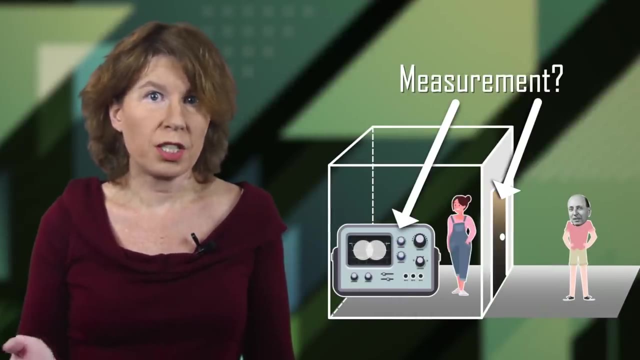 seems to be subjective. Now it's rather obvious what's going on, namely that one needs to specify what physical process constitutes a measurement. Otherwise the prediction is, of course, ambiguous. Once you have specified what you mean by measurement, Alice will either do a 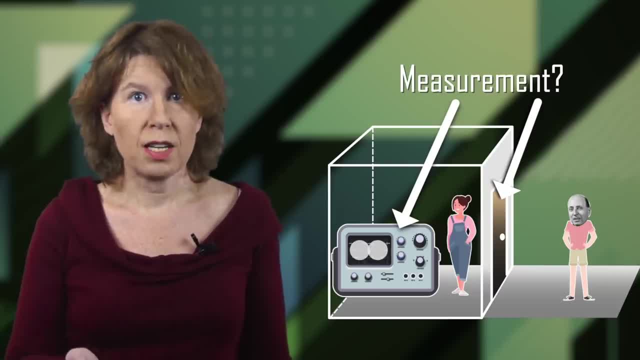 measurement in her laboratory or not, but not both. And in a real experiment rather than a thought experiment. the measurement happens when the particle hits the screen, And that's that. Alice is, of course, never in a superposition, and she and Wigner agree on what's objectively real, If that's. 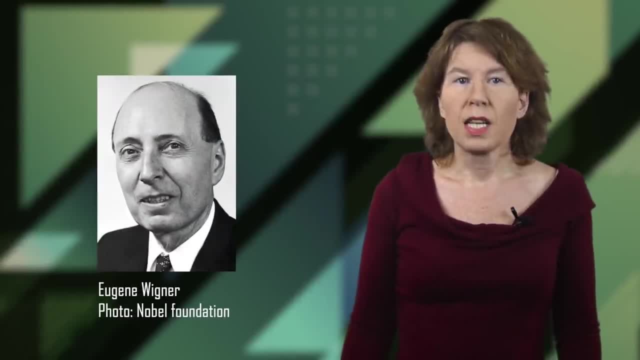 obvious. then why did Wigner worry about it? Because in the standard interpretation of quantum mechanics, the update of the wave function isn't a physical process. It's just a mathematical update of your knowledge, which you do after you've learned something new about the system. 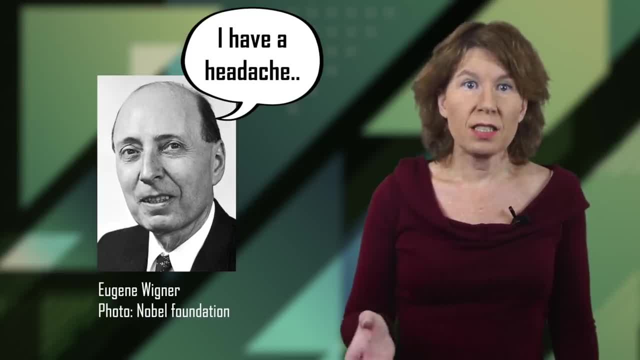 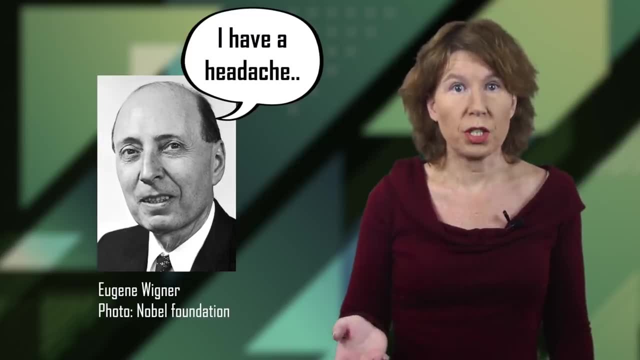 It doesn't come with any physical change. And if Alice didn't physically change anything, then according to Wigner she must indeed herself have been in a superposition. Okay, so that was Wigner's friend in the 90s. 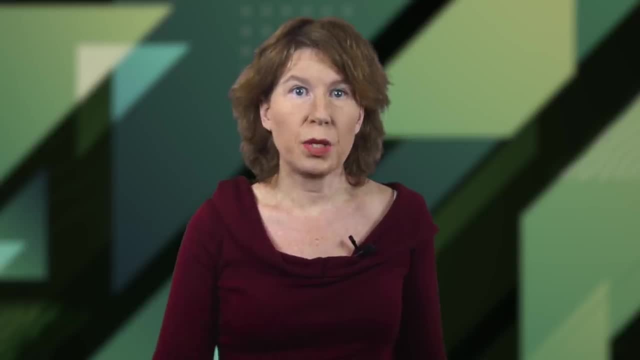 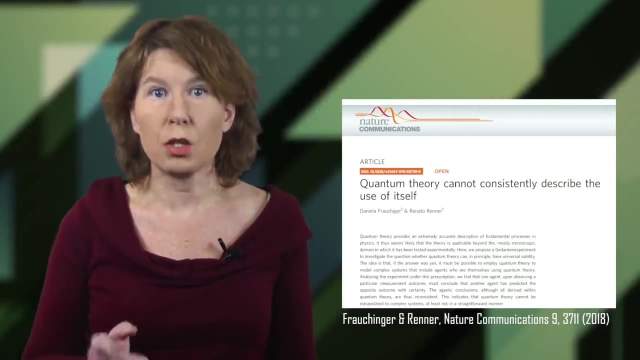 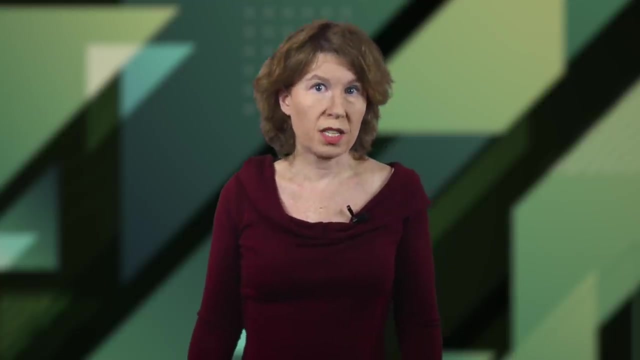 You can't experimentally test this, but in 2016, Daniela Frauchinger and Renato Renner proposed another thought experiment that moved physicists closer to experimental tests. This has been dubbed the extended Wigner's friend scenario. Before we talk more about Wigner and his friends, I want to thank our sponsors on Patreon. 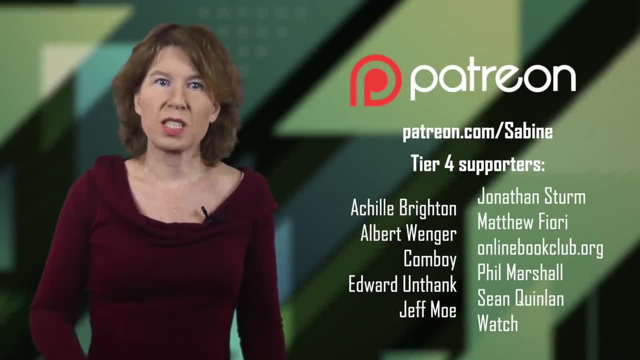 especially our TF4 supporters. Your help is so important to keep this channel going, And you too can help us. Go check out our Patreon page or click on the join button right below this video. Now, what's with the extended Wigner's friends? 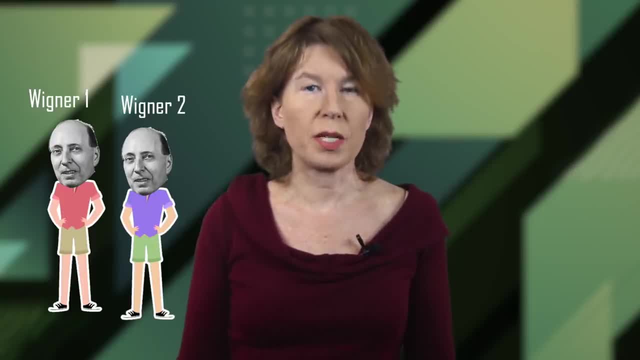 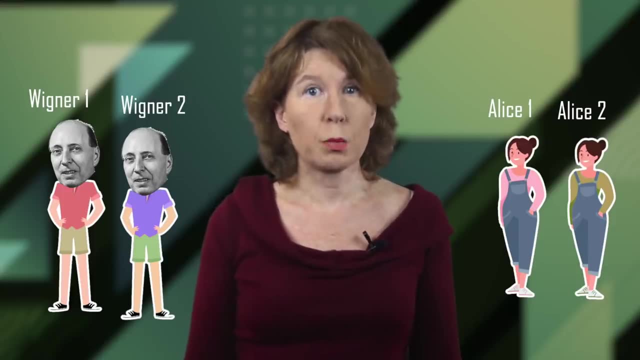 In this thought experiment, you have two Wigners, each of whom has a friend. We'll call these the Wigners and the Alice's. The Alice's each measure one of a pair of entangled particles. As a quick reminder, entangled particles share some property, but you don't know which. 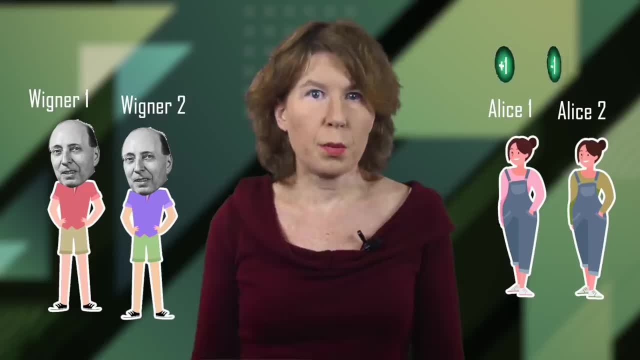 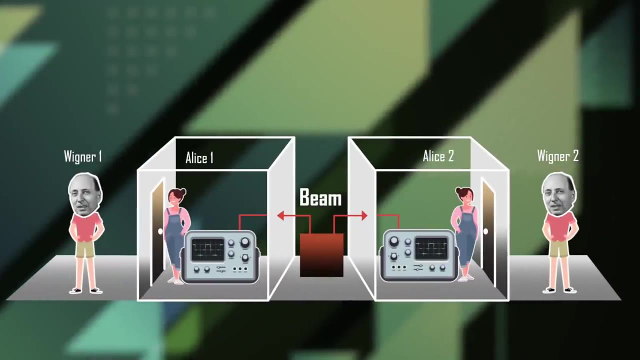 particle has which share. You may know, for example, that the particle spins must add up to zero, but the left particle has spin plus one and the right particle spin minus one, or the other way around. So the Alice's each measure an entangled particle. Now the thing with entangled particles is that if 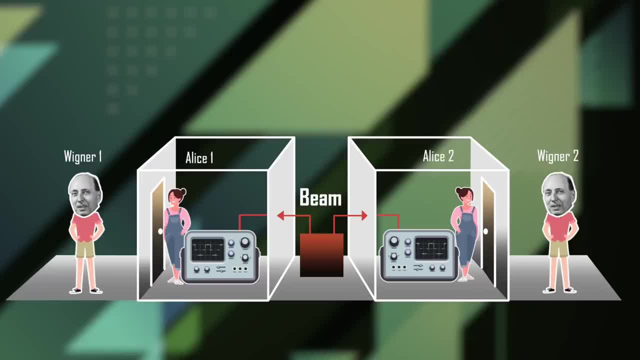 the Alice's measurements don't collapse, the wave function. then now the two Alice's are entangled. Either the left one thinks the spin was up and the right one thinks it's down, or the other way round. And then there's the two Wigners, each of which goes to ask their friend something about. 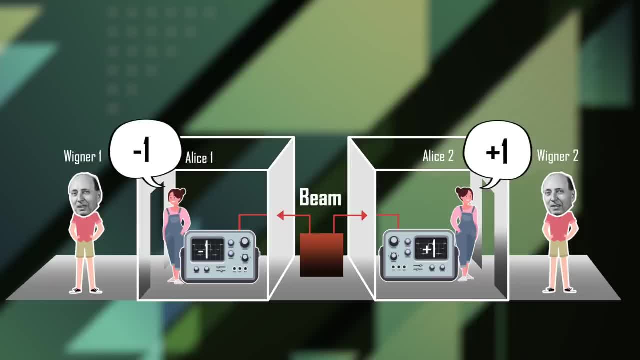 their measurement. And then there's the two Wigners, each of which goes to ask their friend something about their measurement. Formally, this asking just means they do another measurement. Frauchinger and Drenner then show that there are combinations of measurements in which the two Alice's cannot agree with the two Wigners. 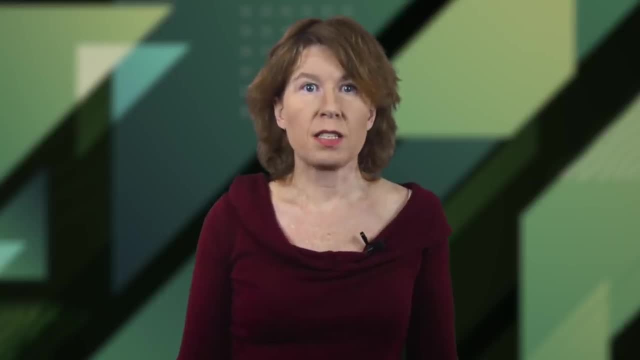 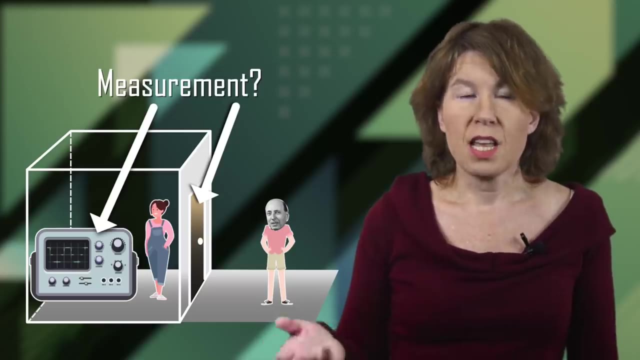 on what the measurement outcomes were. Again, the obvious answer to what happens is that the Alice's either measured the particles and collapsed the wave function, or they didn't. If they did, then their measurement result settles what happens. If they didn't do it, then it's the 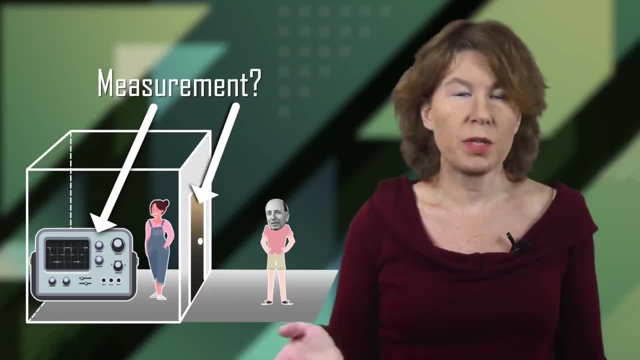 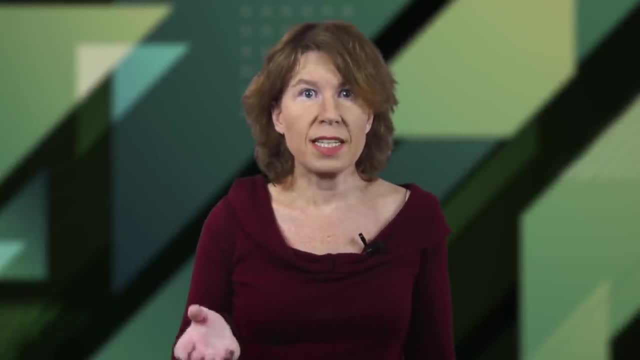 Wigner's results, which settle the case, Or some combination thereof, depending on who measures what. Again, this is only problematic if you think that a measurement is not a physical process, Which is insanity, of course, but that's indeed what the most widely held interpretation of 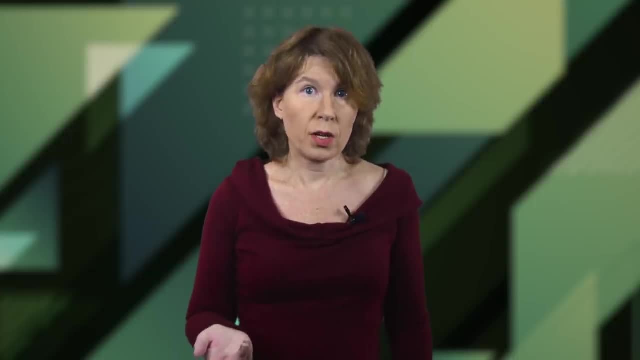 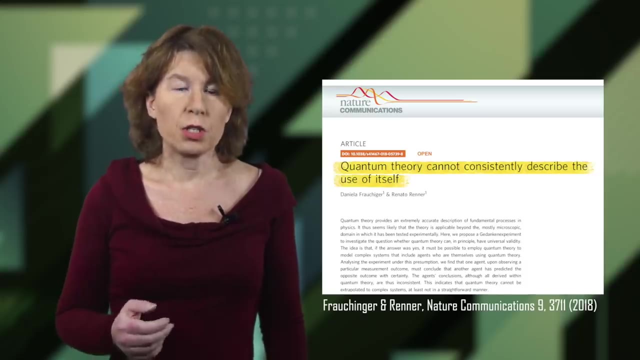 quantum mechanics says, And so Frauchinger and Drenner conclude in their paper that quantum mechanics cannot consistently describe the use of itself, Because you run into trouble if you're one of the Wigners and try to apply quantum mechanics to understand how the Alice's used. 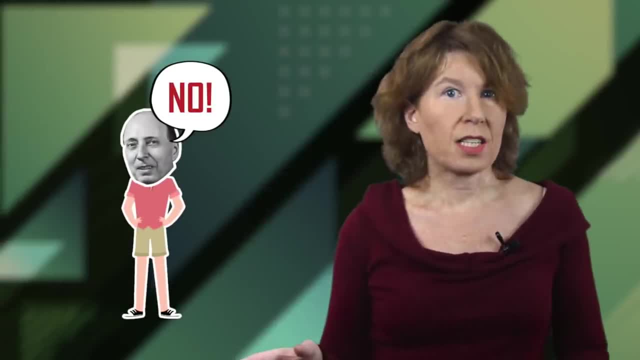 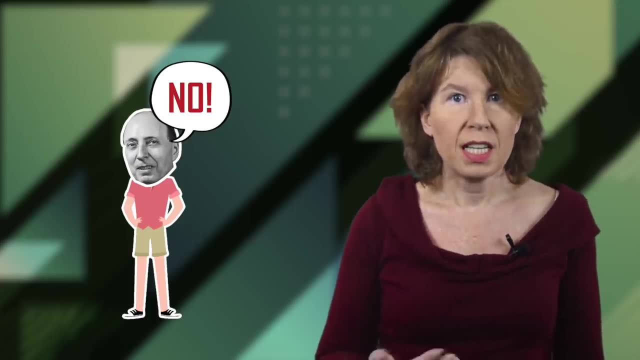 quantum mechanics. You may find this rather an academic argument, But don't get fooled: this innocent sounding statement is a super important result. Historically, internal inconsistencies have been the major cause of theory-led breakthroughs in the foundations of physics. So we're onto something. 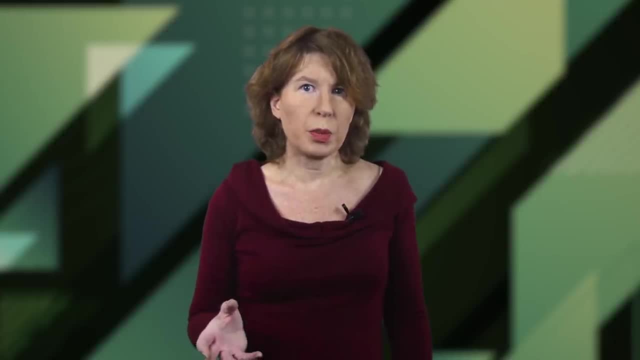 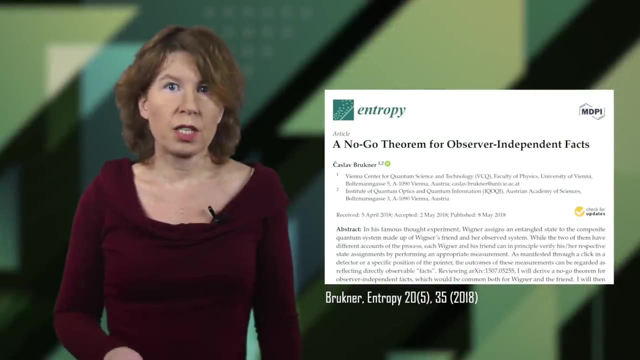 But the Frauchinger and Drenner paper is somewhat philosophical because they go on a lot about what knowledge you can have, about other people's knowledge. But in 2018, Czeslaw Bruckner looked at the problem from a somewhat different perspective. 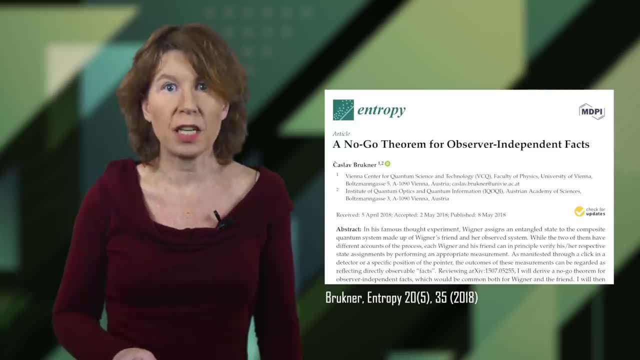 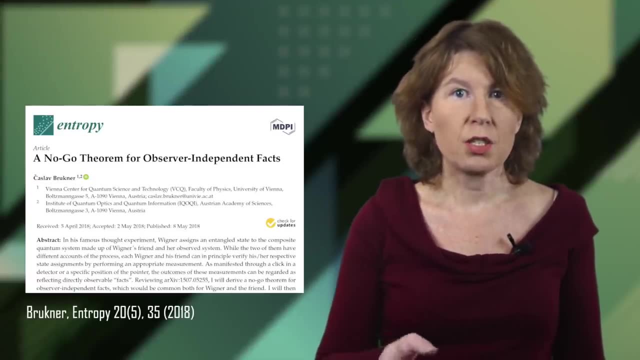 and derived a no-go theorem for observer-independent facts. His formulation allows one to use the measurement of certain correlations in measurement outcomes to demonstrate that the observers in the extended weakness front scenario actually had measurement results which disagree with each other. If that was so, there would, in certain cases, be no observer-independent facts. 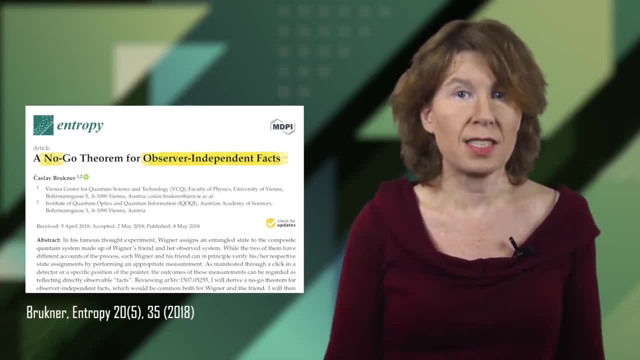 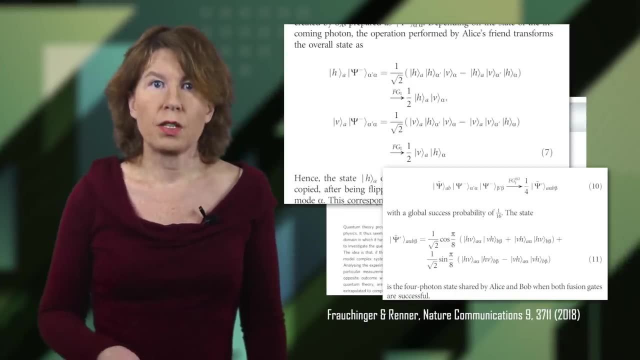 This is the origin of all the talk about objective reality not existing and so on. And yeah, it's really just linear algebra. there aren't even differential equations to be solved. I assure you, I'm not saying this to be condescending or anything. I just mean to say this isn't. 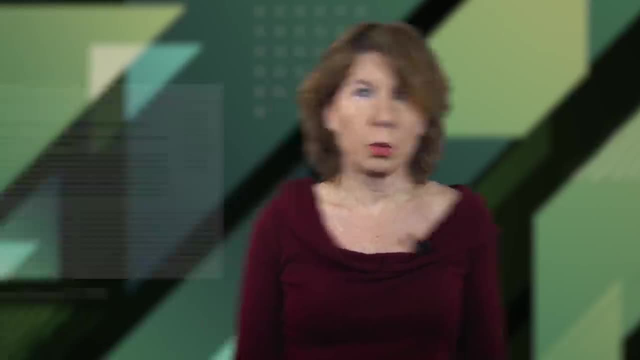 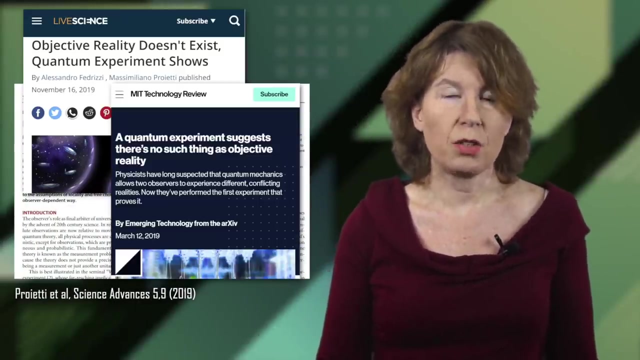 rocket science. Finally, in 2019, a group from Edinburgh actually measured those correlations which Bruckner calculated. That's the experimental test which the headlines are referring to. Now you may wonder who in Edinburgh played the role of the two ellipses and the two weakness. 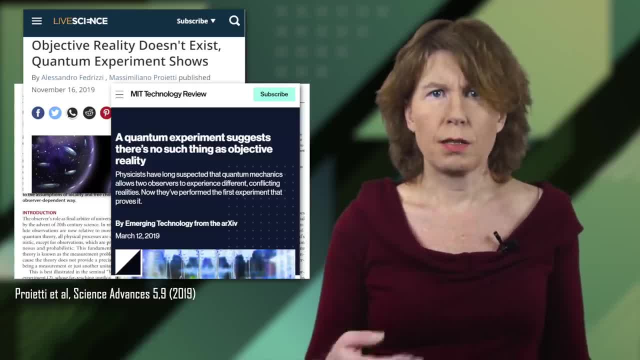 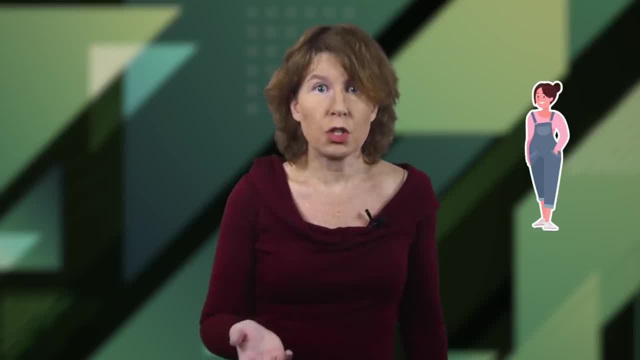 How did the ellipses feel while they were in a superposition? Did the weakness see any wave functions collapse? Well, I'm afraid I have to disappoint you, because the two ellipses were single photons and the two weakness were photodetectors. That's okay, of course. I mean, some of my best friends are photons too- But of course an interaction with a single photon is not a superposition. A single photon doesn't constitute a measurement. We already know this experimentally. A measurement requires an apparatus big enough to cause decoherence. 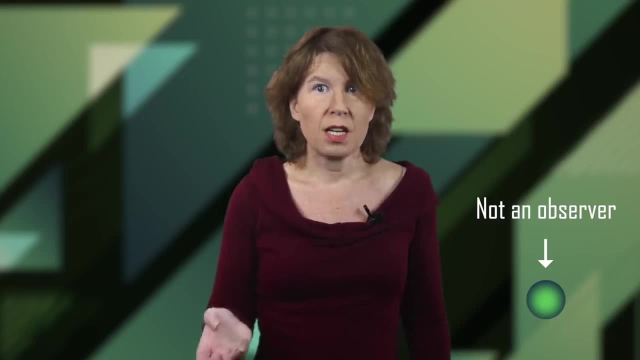 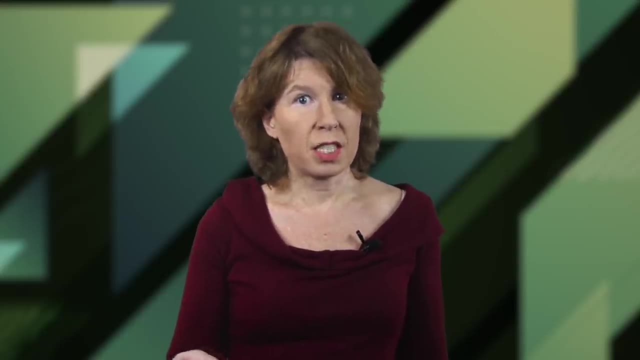 If you claim that a single photon is an observer who makes a measurement, that's not just a fanciful interpretation, that's nonsense. The alleged mystery of all those arguments and experiments disappears once you take into account that a measurement is an actual physical process. But Since quantum mechanics doesn't require you to measure a single photon, you can't measure a single photon. There is no way to define just what this process is. You can make contradictory assumptions about it, and then more contradictions follow from it. 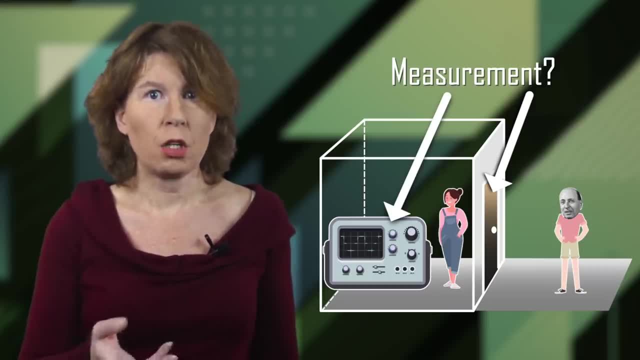 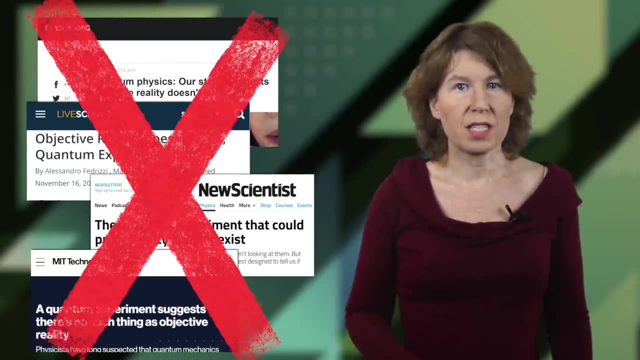 It's like you have assumed that zero equals one and then show that a lot of contradictions follow from it. So, to summarize, no one has proved that reality doesn't exist and no experiment has confirmed this. What these headlines tell you instead is that physicists slowly come to see that quantum 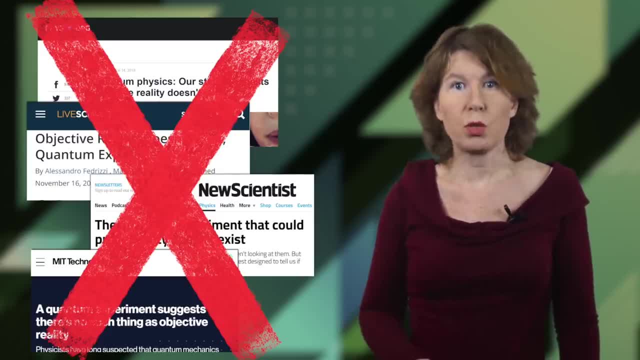 mechanics is internally inconsistent and must be replaced with a better theory, And that's what I'm trying to say. If you find a theory, one that describes what physically happens in a measurement, And when they find that theory, that will be the breakthrough of the century. 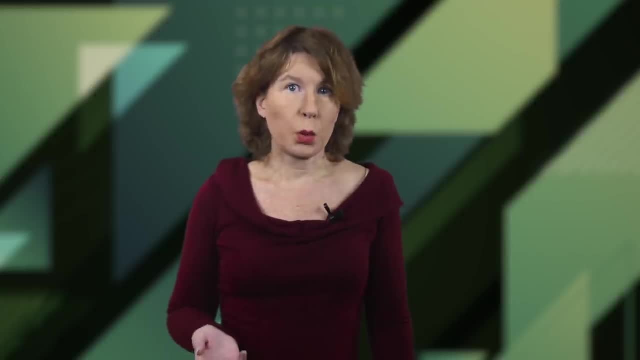 This video was sponsored by Brilliant. I wasn't kidding when I said quantum mechanics isn't rocket science. It's really mostly linear algebra and not remotely as incomprehensible as most physicists want you to believe. If you want to understand quantum mechanics in more depth, Brilliant is a great starting. 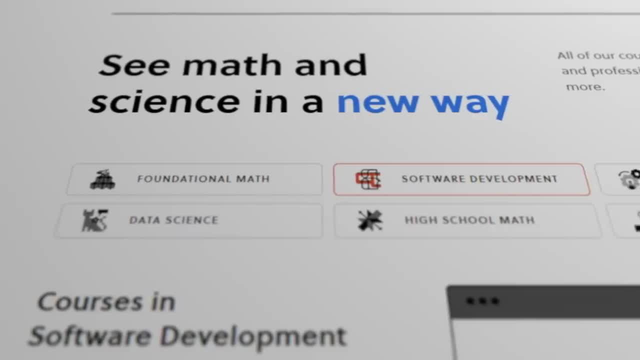 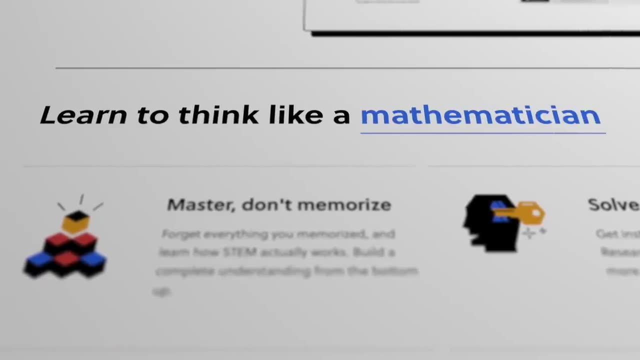 point. Brilliant is a website and app that offers courses on a large scale. If you want to understand quantum mechanics in more depth, Brilliant is a great starting point. It offers courses on a large variety of topics in science and mathematics. Whether you want to learn something new or freshen up your knowledge, Brilliant is a 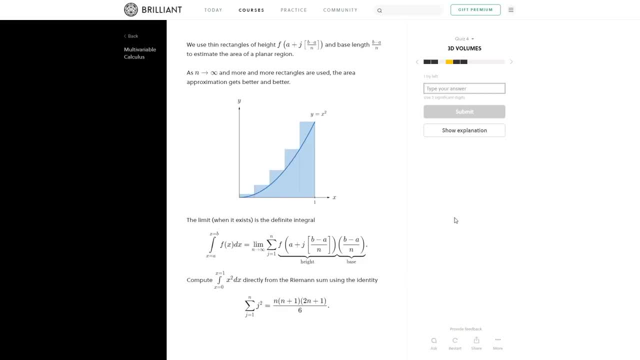 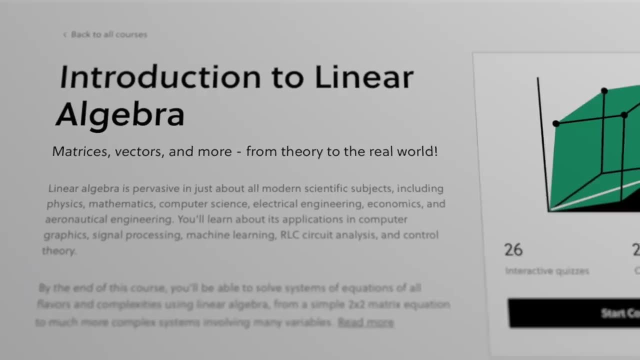 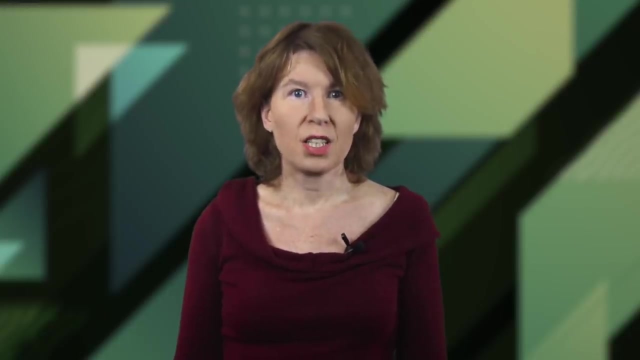 simple and fun way to do it. All their courses are interactive, so you are challenged with questions and can check your understanding along the way. For this video, for example, I recommend their courses on linear algebra and quantum objects. To support this channel and learn more about Brilliant, go to brilliant dot org. slash sabine.